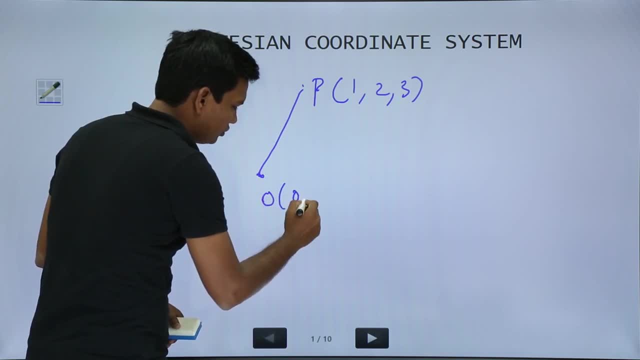 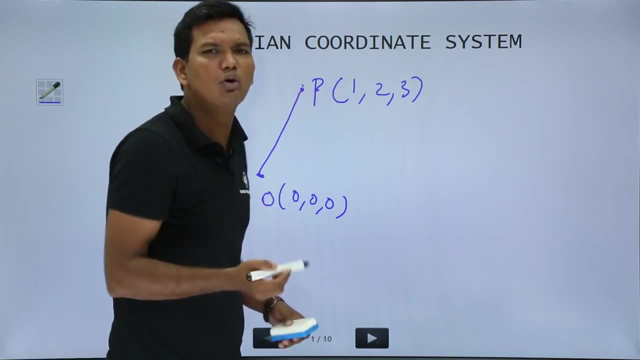 coordinate of origin. Origin coordinate would be nothing but 0,, 0, 0, right. What do you mean by this? When you say any point is 1,, 2,, 3, it means nothing, but it is 1 unit away from the x. 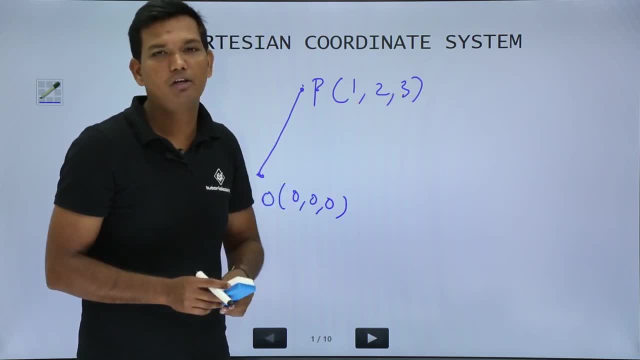 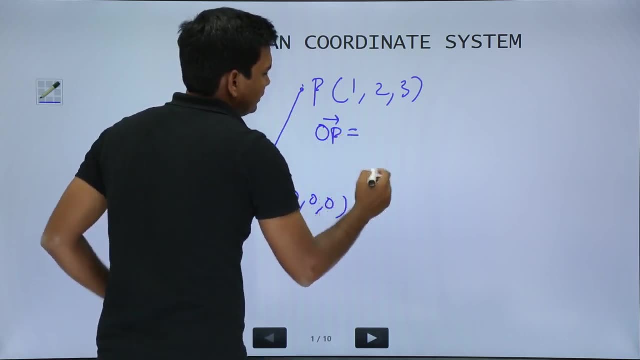 axis, 2 unit away from the y axis and 3 unit away from the z axis, right. So if you want to write the vectored form, this would be nothing but OP vector. let me call it. It will be nothing but 1. 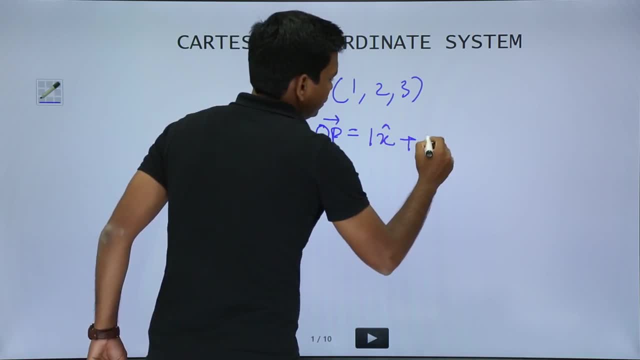 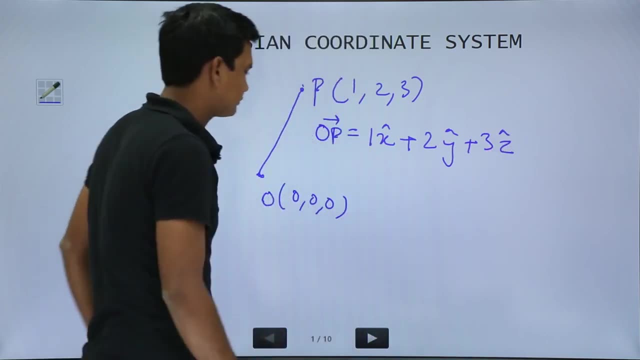 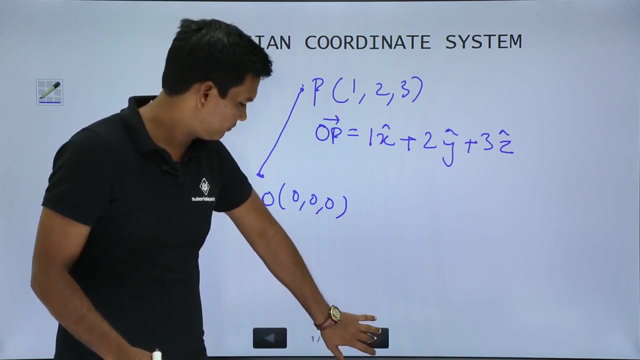 x cap plus 2 y cap and 3 z cap. So this is how it will look like. Now let us look into the figure and try to understand more on this. So this is some- I have drawn some of this figure. Let us try to. 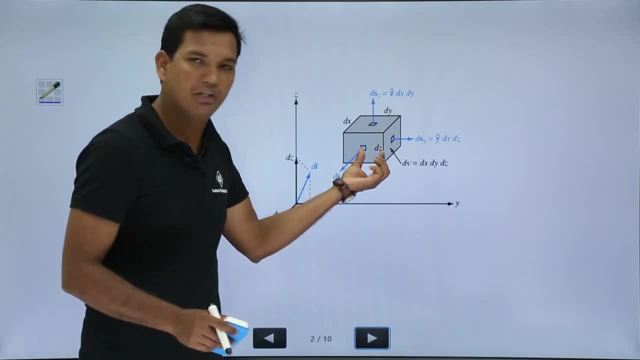 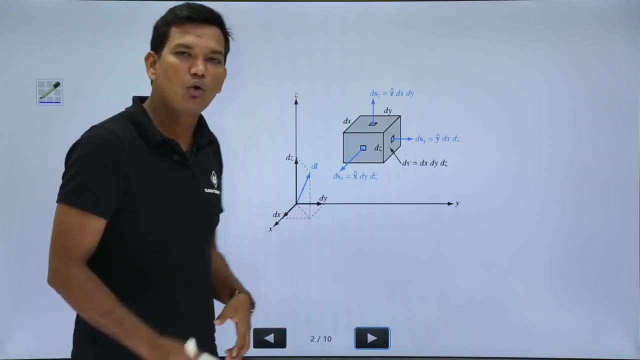 understand this. Now, it is just a cube here, right, Which is nothing. but this is my y axis, z axis and this is my x axis, okay, So if I have drawn a cube, see whenever I want to try to find it out. area- area is also a vectored quantity, right? Remember? 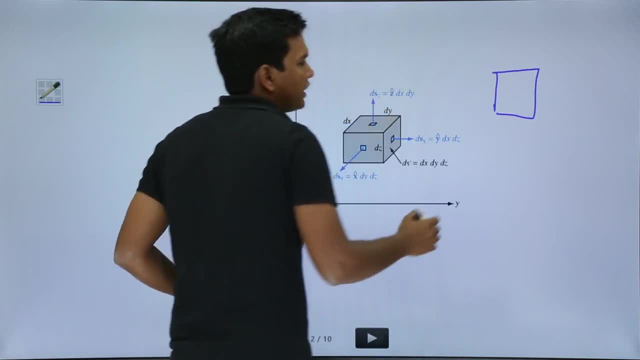 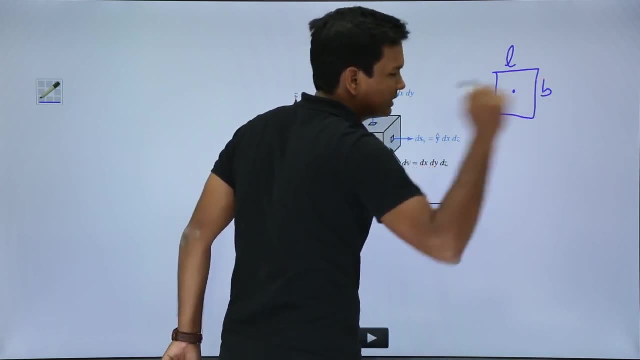 if this is nothing, but your some square when you try to find it out, the area which will be nothing but length into breadth, but there will be a unit vector which will be pointing outward to this board. right, So this will be like this. okay, Same way if you look here to this side, if you 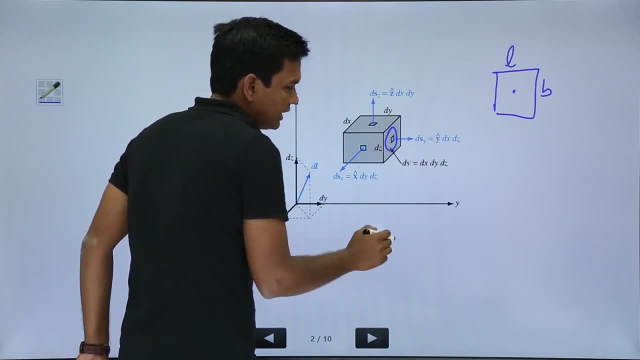 look right, The area, the ds, is nothing but the area. it is in which plane. Basically, this is going this side, So which is, if I look, that is the area right. So this is the area right, So. 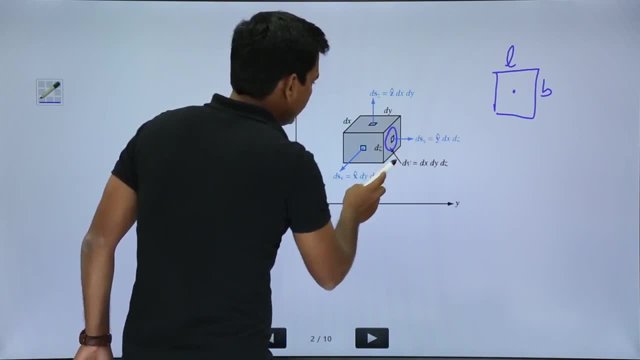 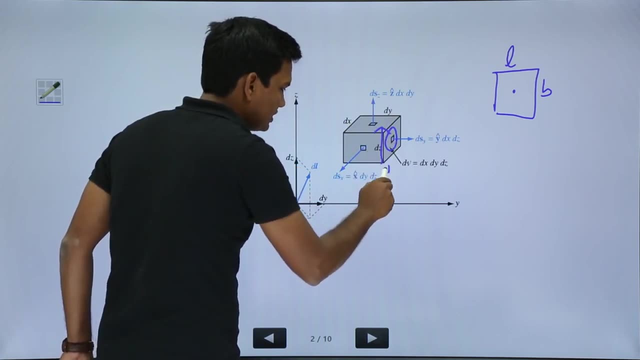 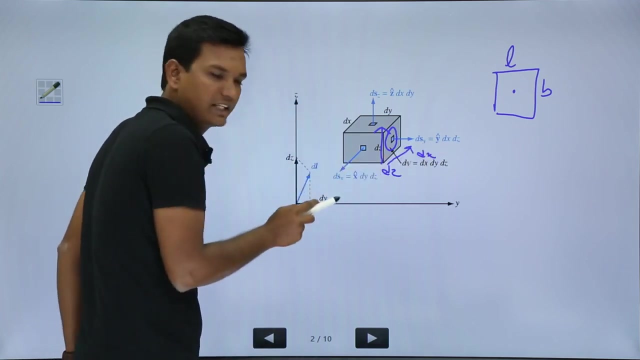 that, if I look, this, which is nothing but your dx right, And another is nothing but your dz right. So this part which is going up is nothing but your dz. that part which is nothing but your x axis will be your dx right, Which is nothing but the variation along the x axis right. So 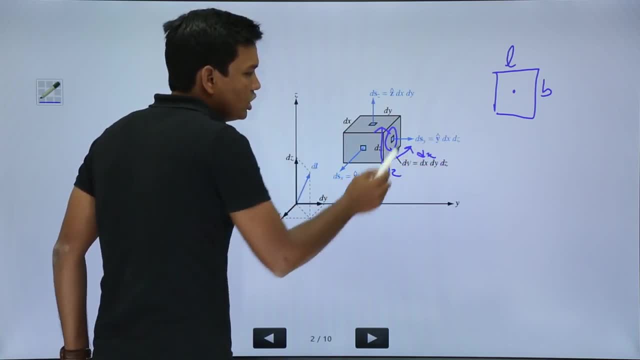 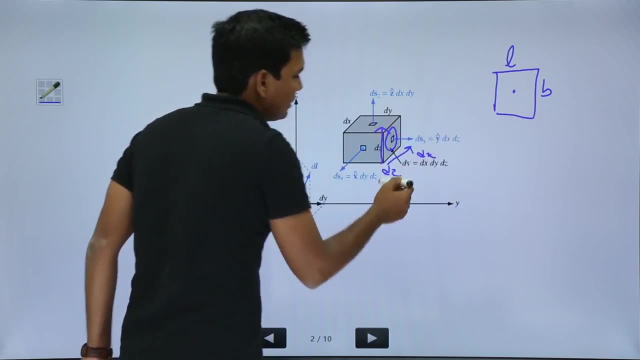 this is variation along the z. this is variation along the x. So when you take the area of this plane, there will be another vector generated which will be perpendicular to this plane, which is nothing but your y cap. you can see that here, right? So if I rub this, you can understand.